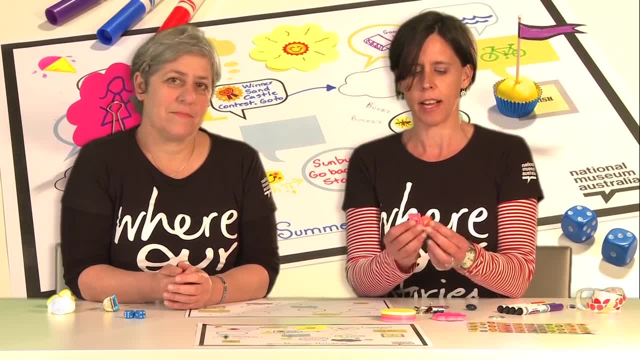 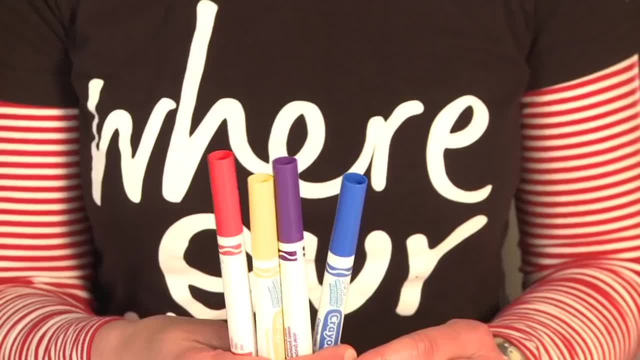 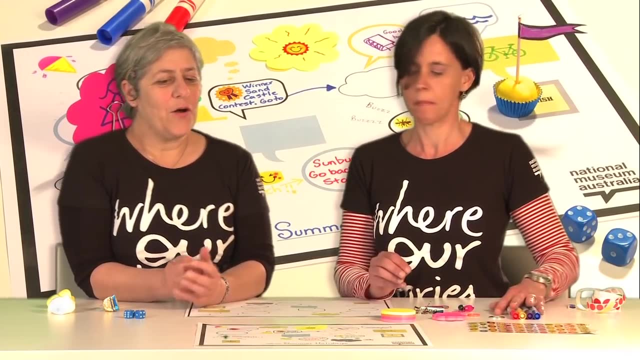 or just beads and buttons that you might have around home too. Don't forget those textures, Kelly. Bright coloured textures are always good to decorate your artwork or your board game with Kelly. Yes, Amanda, If we're going to make our own board game. 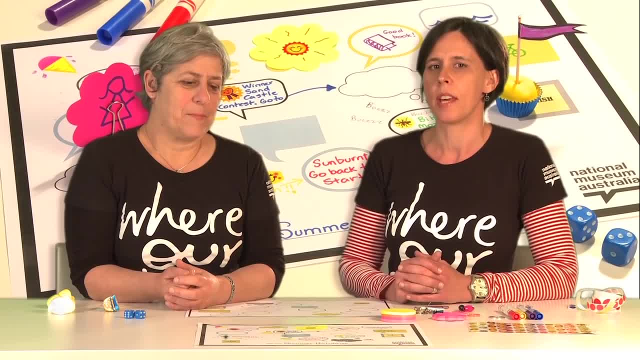 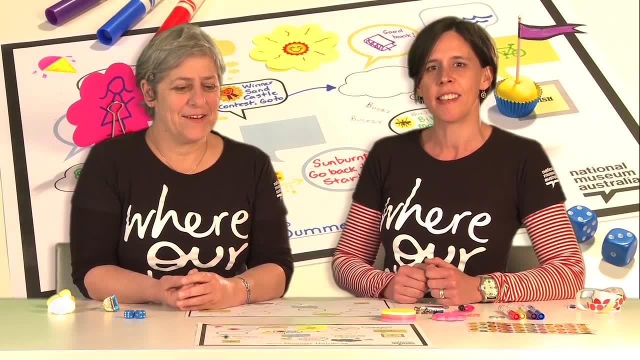 we have to come up with a theme. Yes, What's a good theme? I know We all love going on holidays. Let's do a Summer Holidays in Australia. board game- Great idea. Do you think we should label this game? Yes, definitely. 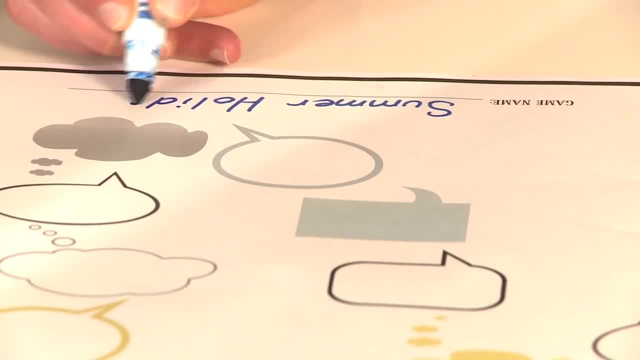 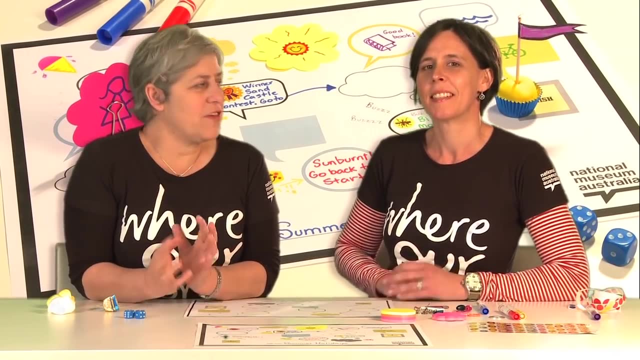 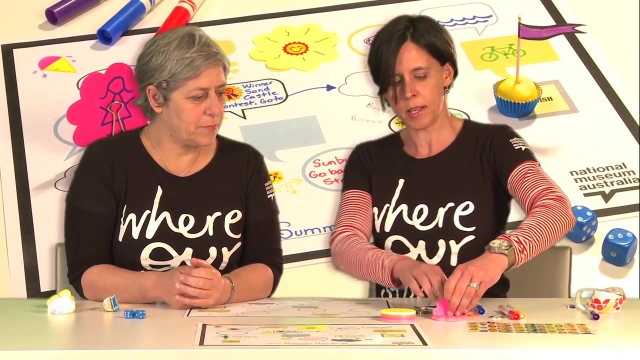 Summer Holidays: Summer Holidays. But, Kelly, before we get started, I think we need to make some game pieces. Yes, some game characters to move around the board. Yes, I know I'm going to make a little game piece out of this post-it note. 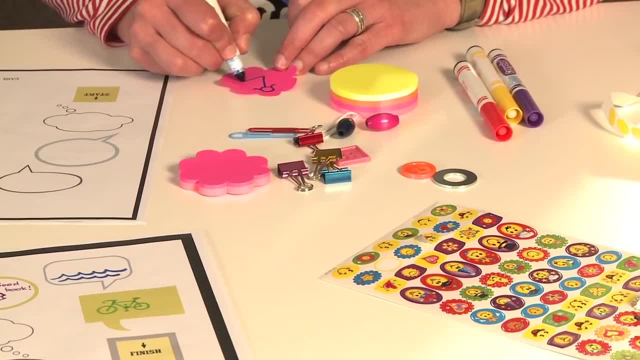 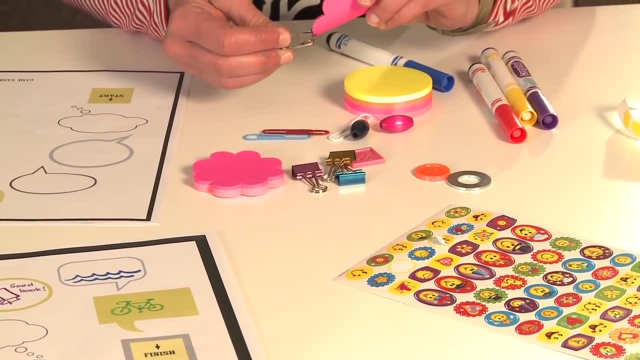 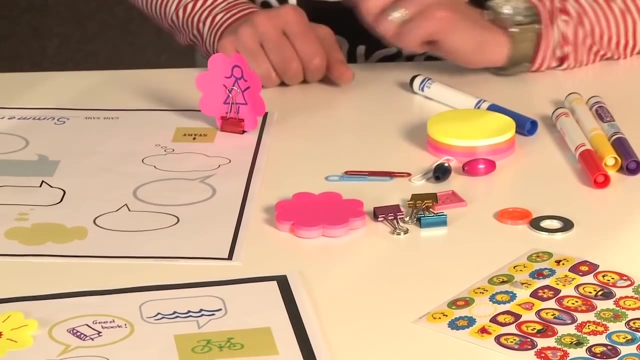 I'm going to draw me on it And to make it stand up, I'm going to use one of these bulldog clips And if you fold it up, you get a flat bottom And you can stand your character. That's fantastic, Kelly. 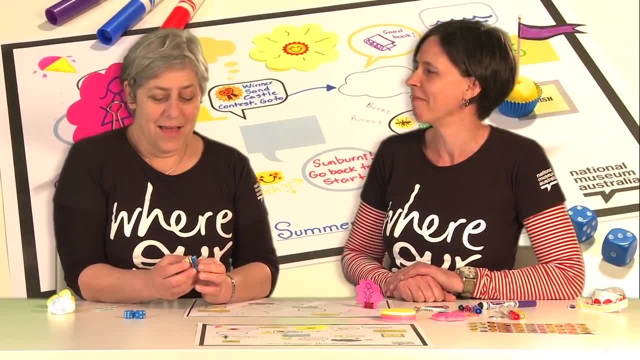 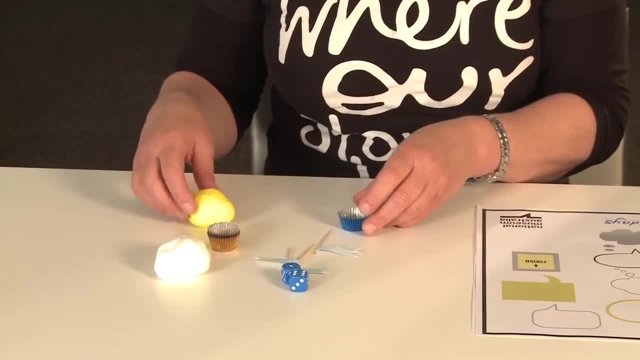 Now, Kelly, you know I like cooking. I do. I searched my cupboard and I found lots of these tiny foil cupcake pins. They're cute. I'm going to use one of them. a little bit of modelling clay, Roll it up. 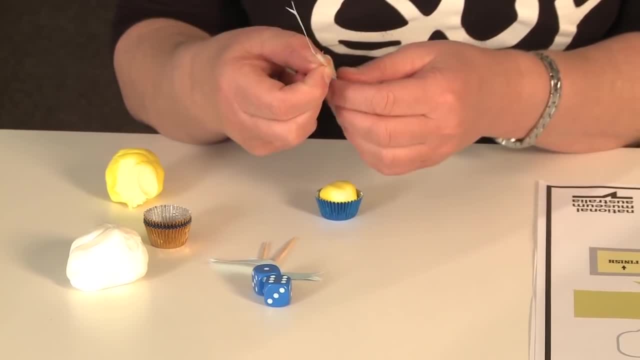 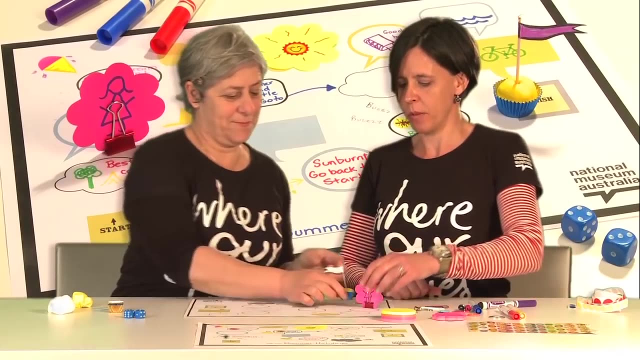 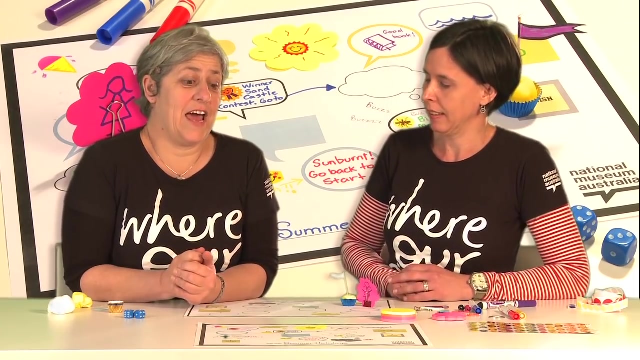 Place it in there. And then, because I love decorating my cupcakes, I have lots of flags That looks great. There's my game piece. That looks good. We're ready with our game pieces. Something's missing. Yeah, I think we need to decorate our game board. 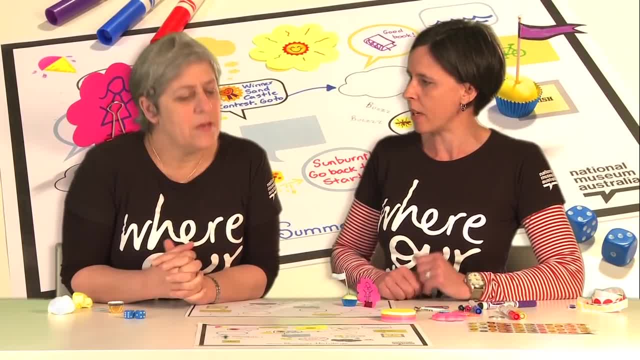 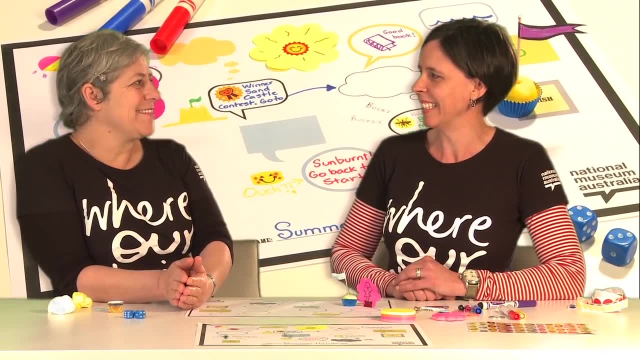 We do. We need to have rules or challenges that we can play with. What's something that isn't good? that happens on a summer holiday Sunburn- Nobody likes to get sunburned. No, no, no. That needs to be a rule. 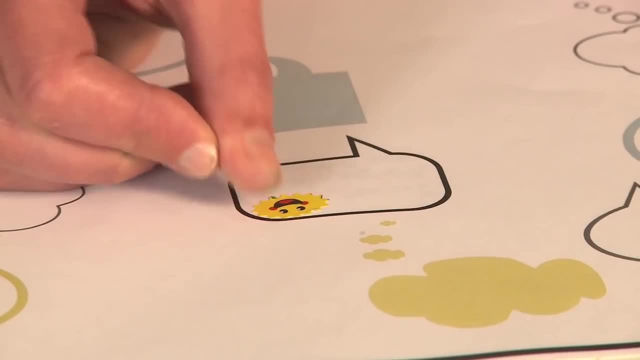 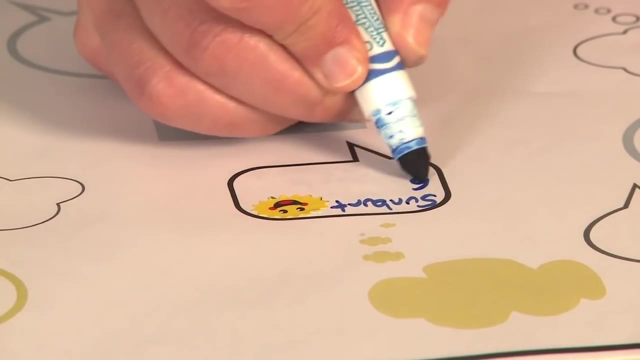 I'll put a little sticker here. I've got a little sun Sunburned. What's going to happen if you get sunburned? Go back two paces. I reckon you should go back to the start, Oh me. 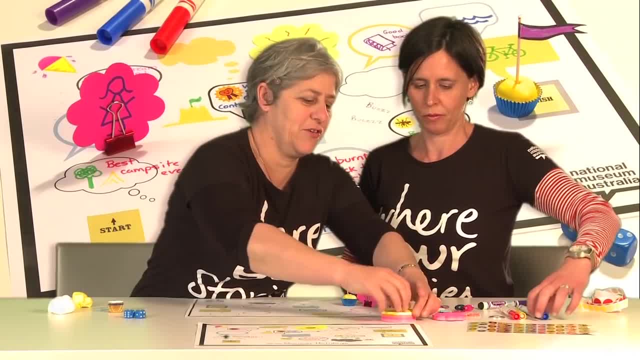 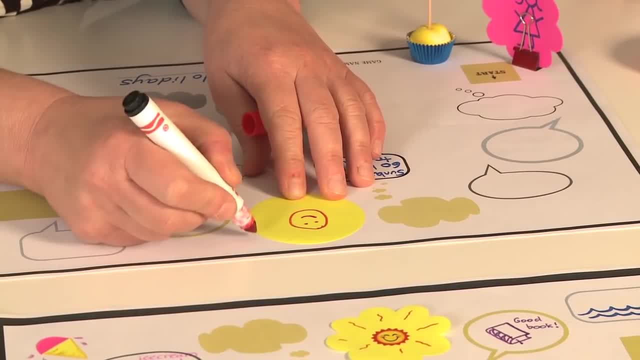 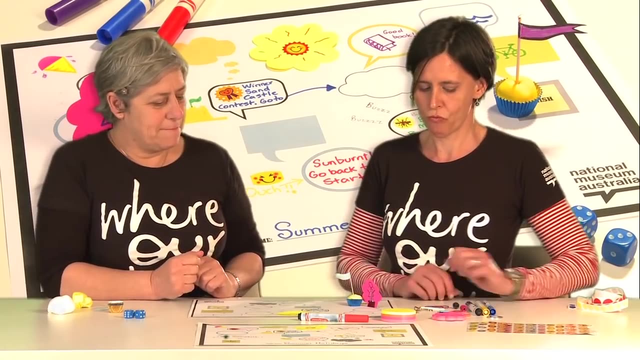 Go back to start. I love it. I think, Kelly, we should draw a sun too. Yeah, definitely, There we go. Keep it simple: Big smiley face and lots of rays, Yeah, cool. OK, We need something to move the game forward. 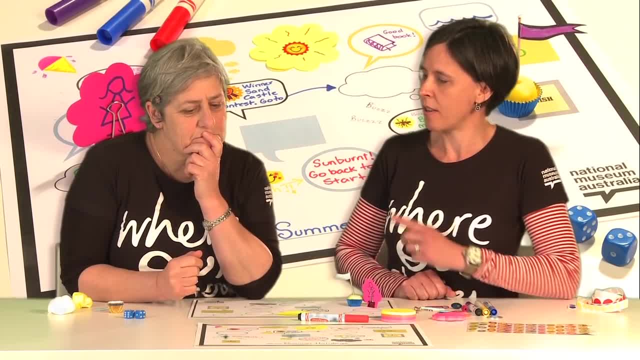 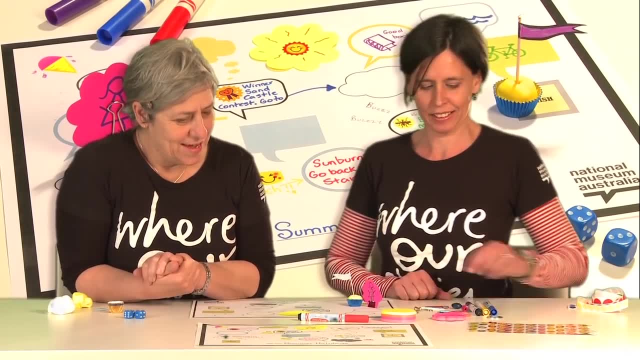 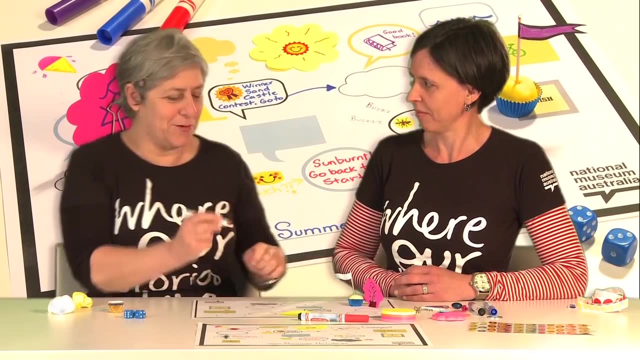 Another idea. I know Something good that can happen. You can win the sandcastle building competition at the beach. I love sandcastles. So how many paces should we move forward? Three, Three, Terrific. Oh, you're asking me to draw. 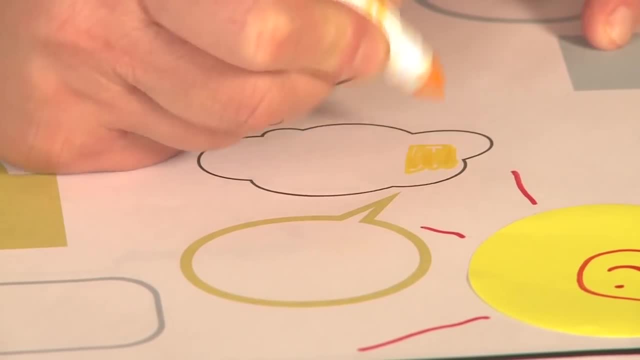 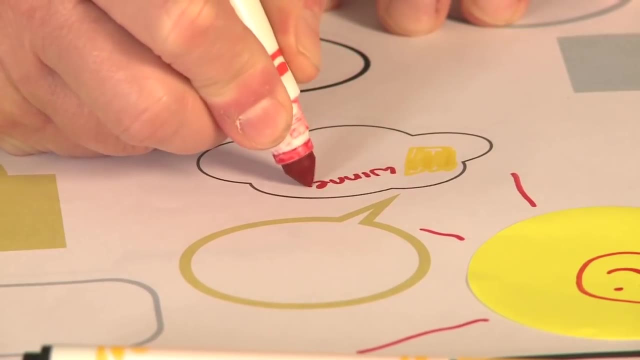 Here's my sandcastle. I've got a little metal sticker here too. It's a winner, Winner, Go forward. Three, Three, Great Amanda. I hate being bitten by mozzies when I'm on holidays. I reckon that needs to be part of the game. 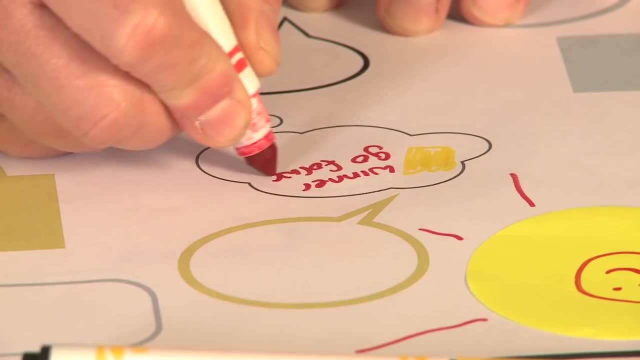 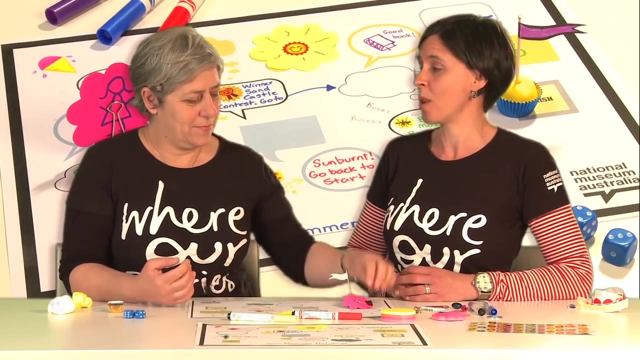 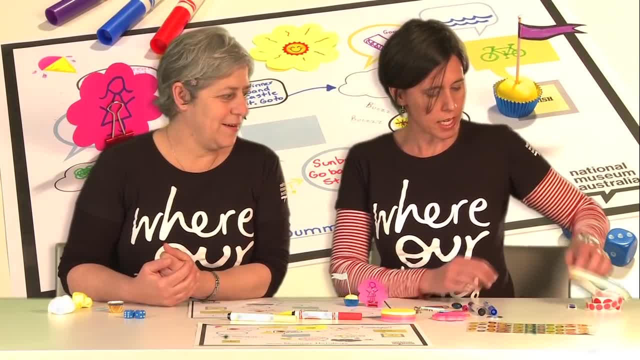 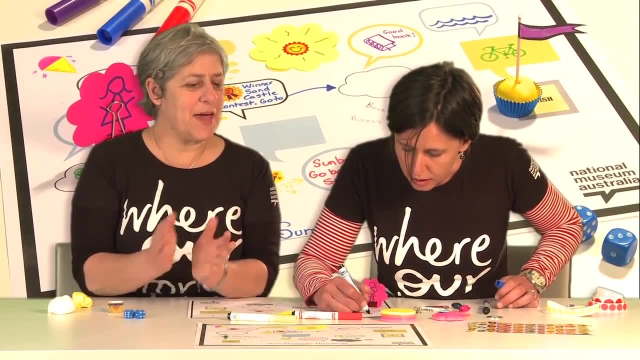 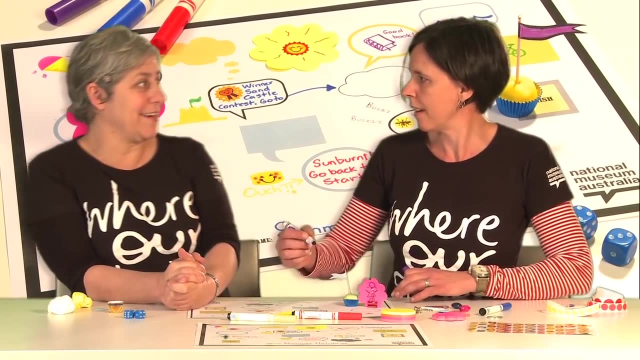 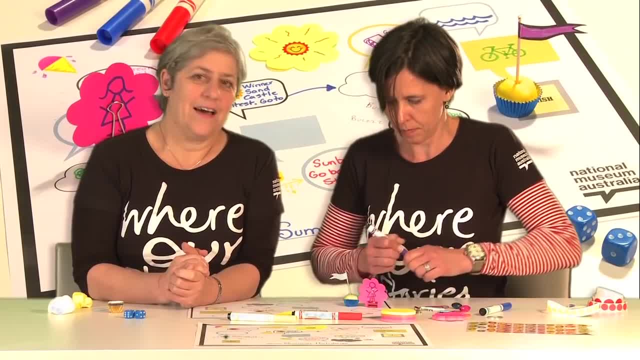 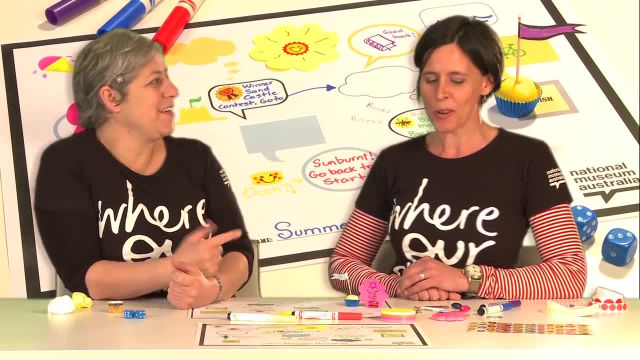 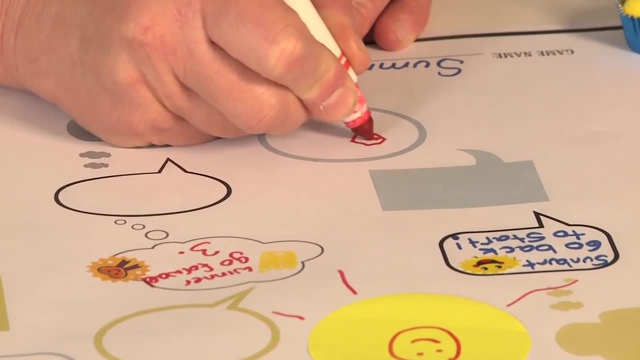 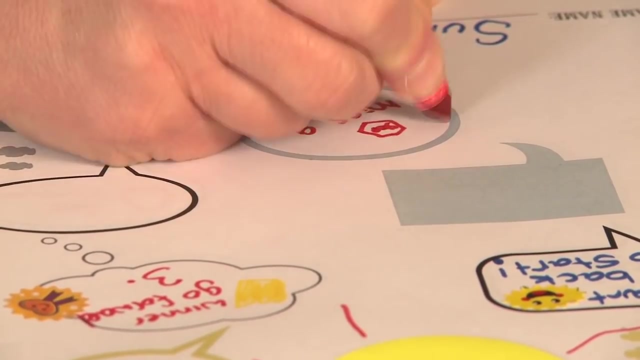 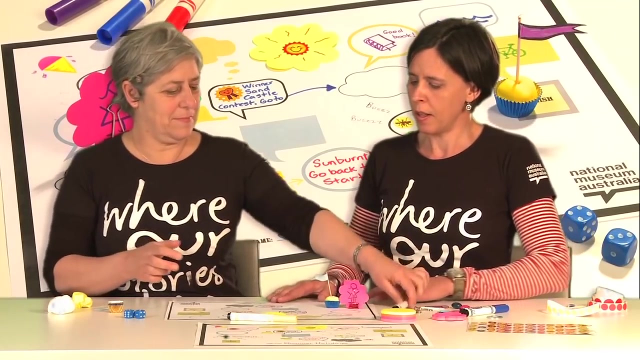 Spot. I've got another idea. What's that? Stop Ice cream van. Yay, of course, Miss a turn. You have to have ice cream vans on the holidays. Stop, Miss a turn. Ice cream, That's gorgeous. 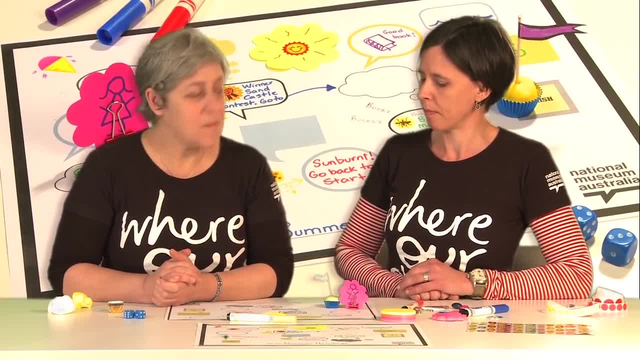 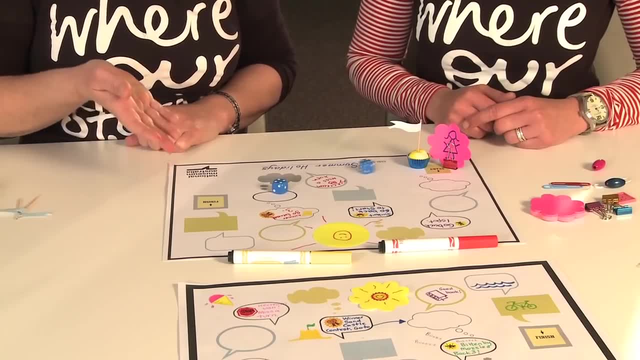 You know what, Amanda? I reckon we're nearly ready to play our game. Shall we get started. We need some dice. Shall we, Shall we. Let's go. Oh, four, My favourite number One. two, three.